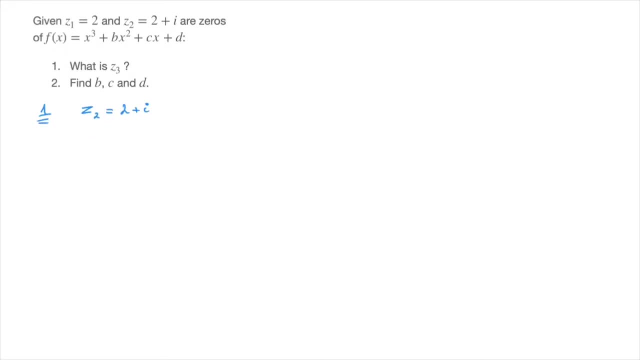 this conjugate zero is one of the zeros of the polynomial function, f of x squared plus i. In other words, since f of 2 plus i equals to zero, this implies, or it tells us, that f of 2 minus i, the conjugate, must also equal to zero. So we can go ahead and state that z3, the third zero, must equal. 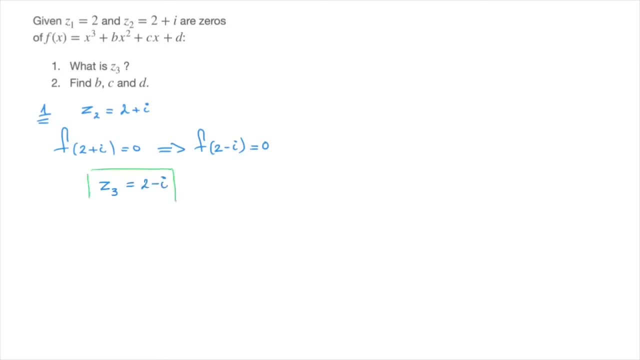 to 2 minus i, And that's the answer to the first question. We now move on to the second question. Remember, we have to find the values of the coefficients b, c and d. I'll just copy this polynomial function to make things a little clearer. 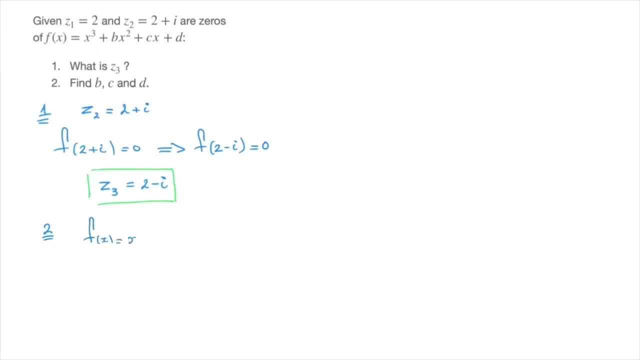 We have f of x, which equals to x cubed plus b, x squared plus c, x plus d. Now the trick for finding the coefficients b, c and d is to write this polynomial in its factored form. Since this is a cubic polynomial, it has three linear factors and because we now know all three of this polynomial, 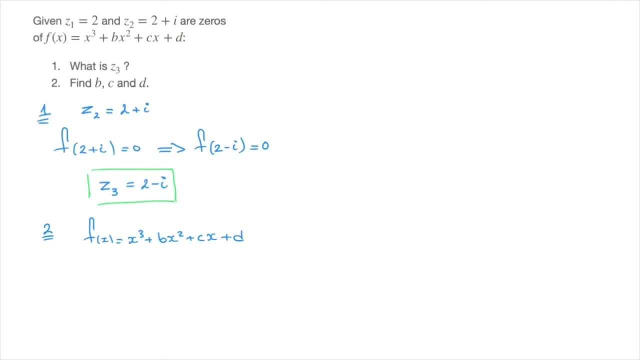 zeros. we have to use this polynomial to find the values of the coefficients f and d To find the. we can go ahead and write this polynomial in its factored form. Indeed, since we know that 2, 2 plus i and 2 minus i are all zeros, 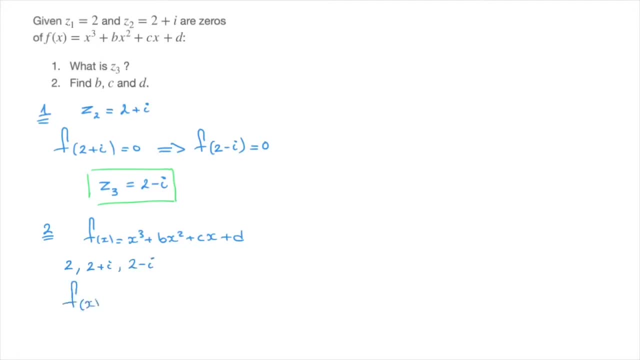 we can go ahead and state that f of x equals to x minus 2,. that's the first zero times x minus 2 plus i. that's the second zero times x minus 2 minus i. that's the third zero. 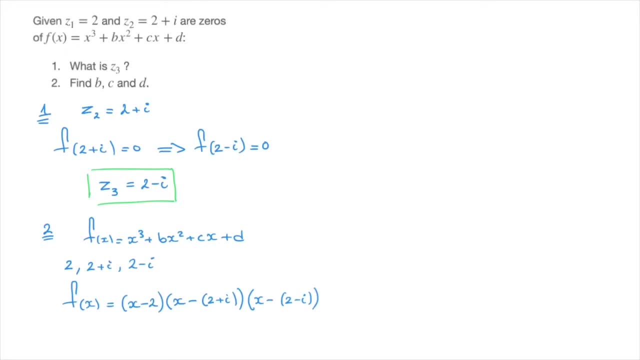 All we have to do now is open up these parentheses and equate the polynomial we get to the polynomial we were given with b, c and d. So let's go ahead and do that. I'll do my working in the upper right-hand side of this page up here. 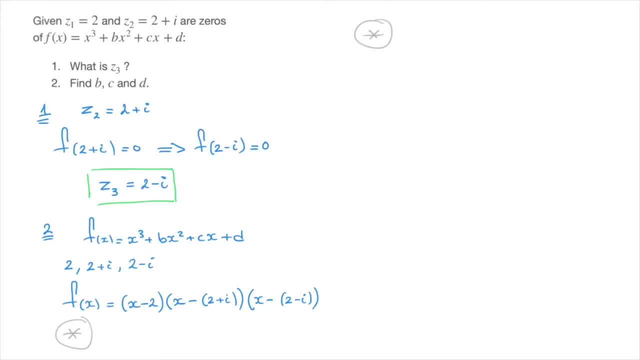 And the first thing I'll do is distribute these two last parentheses. In doing so, we find the following: f of x is equal to x minus 2 times in parentheses, x squared minus 4x plus 5.. And by all means, go ahead and press pause to check.